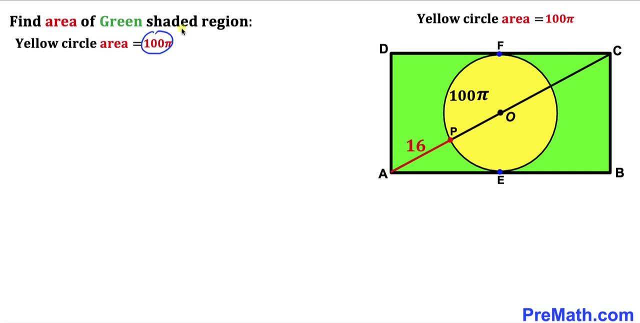 yellow circle is 100 pi and we are interested in calculating the radius of this yellow circle. And now let's recall the area of a circle. formula: area equals to pi R squared, where R is the radius of the circle. Let's go ahead and equate these two equations. So therefore, we are going to get pi R squared equals to 100 pi R squared. 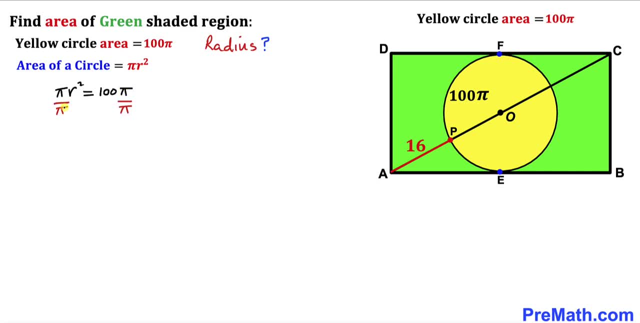 pi. Let's go ahead and divide both sides by pi, So therefore our r square value turns out to be 100.. Let's go ahead and take a square root on both sides to undo this square, So therefore our radius r turns out to be 10 units. So therefore we can see that our this radius op. 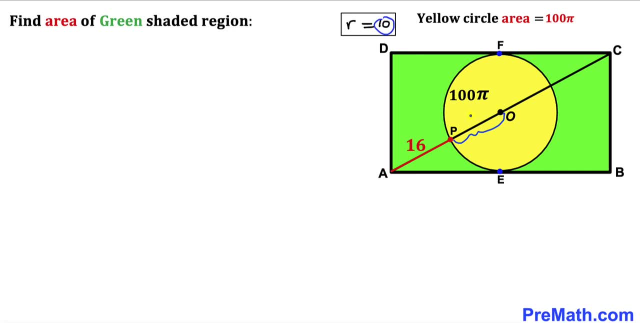 turns out to be 10 units, So I can write down 10 over here. And here's our next step. I have connected these points e and f, and e f turns out to be the diameter of this yellow circle that passes through this center out. And now let's recall the circle theorem, According to: 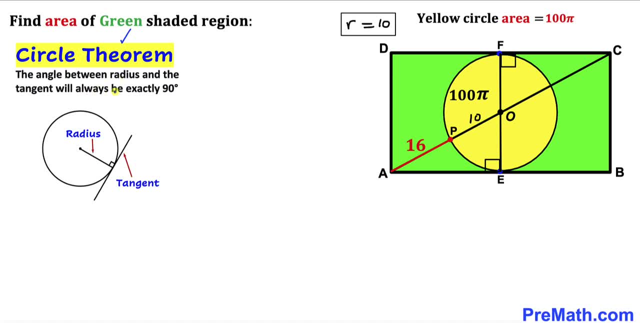 this theorem, the angle between the radius and the tangent line will always be 19.. So this angle is 90 degrees, as you can see in this diagram And here we can see: this is our tangent line and this is our radius and this angle is 90 degrees. So no wonder these, both angles, this angle. 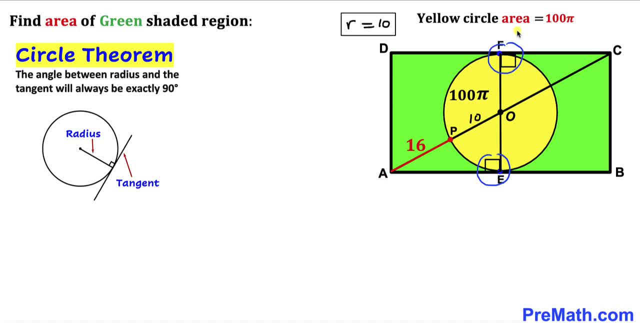 and this angle are going to be 90 degrees each, Since o e and o f are the radii and we can see that this a, b and c d are the tangent lines. So this angle is 90 degrees and this angle is 90 degrees. 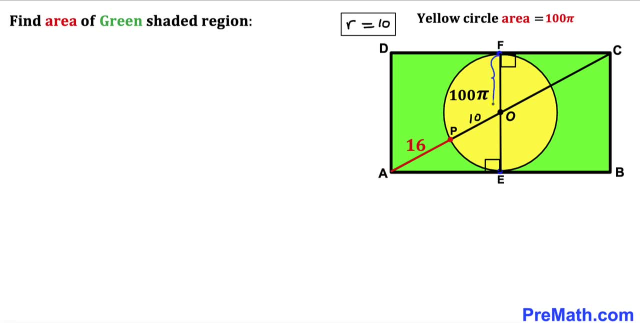 And now let's make an observation. We can see this: o f is the radius of this yellow circle, and we know the radius is 10.. So, therefore, this length is going to be 10 units. Like this, o e is the radius as well, so this is going to be 10 units of. 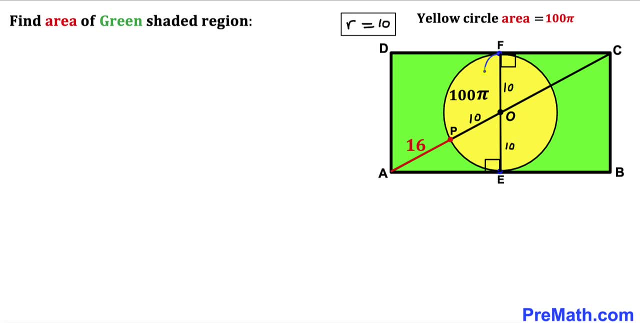 as well. So therefore, this whole diameter e f is going to be 10 plus 10 is going to make 10ies of ek, is going to make 20.. And we can see in this rectangle, this EF length is same as this length, AD. If this is 20, then this AD length is going to be 20 units as well. And here's our next. 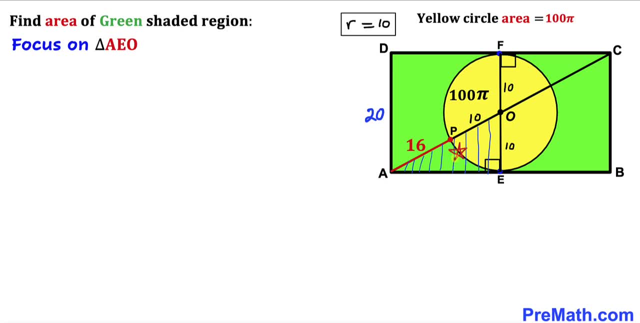 step. Let's focus on this right triangle, AEO, whose this side length, AO is going to be 16 plus 10.. That is going to make 26 units. And now we are going to use the Pythagorean theorem And here's: 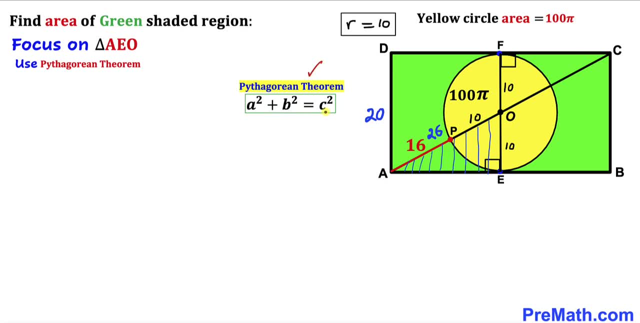 our Pythagorean theorem: A square plus B square equal to C square. Let me call this longest leg as our side C. I'm going to call this side lowercase A and this side lowercase B, And now our task is to calculate this side length A. So let's go ahead. 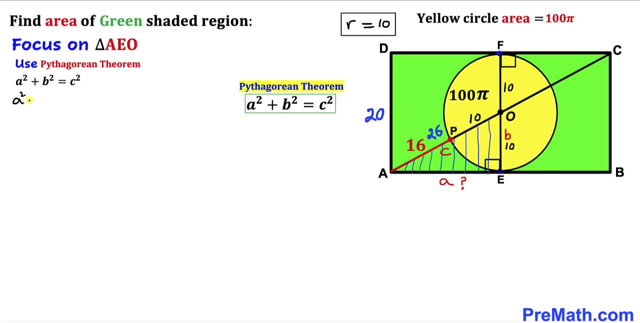 and fill in the blanks in this formula We don't know. A square plus B is 10 whole square equal to 26 whole square. Let's go ahead and subtract 100 from both sides, So this is gone. So A square turns out to be 500.. 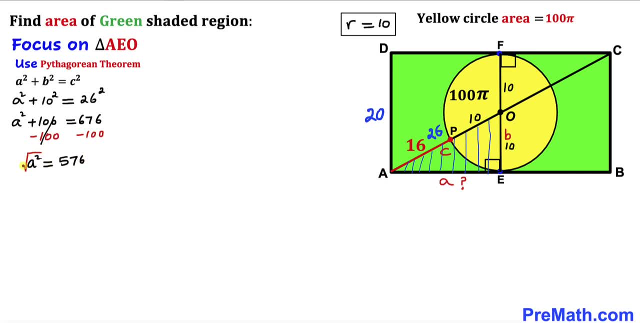 76.. Let's undo this square by taking square root on both sides. So, therefore, our A value turns out to be 24.. So, therefore, our this A length turns out to be 24 units. And here's our next step. Let's 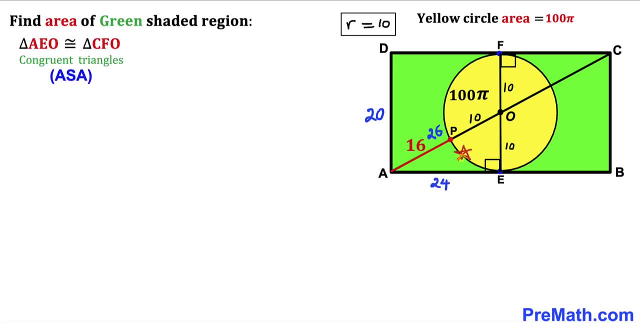 focus on these two right triangles, A, E, O, and this other right triangle, C, F, O. We can see that both of these right triangles are congruent triangles according to angle side angle congruency theorem, Since this side length OF is equal to this side length OE. we know that these 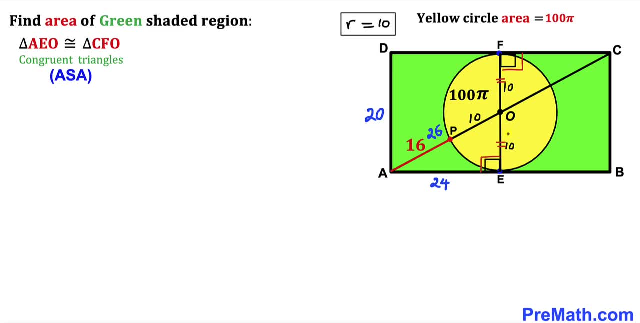 two angles are 90 degree angles. furthermore, these angles are vertical angles and they are congruent. so no wonder both of these triangles are congruent. so therefore we conclude that this side length AE is equal to this side length FC. this is 24 units. so therefore this has got to be 24 units as well.